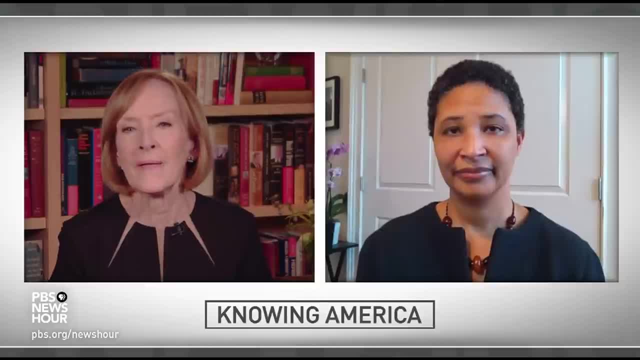 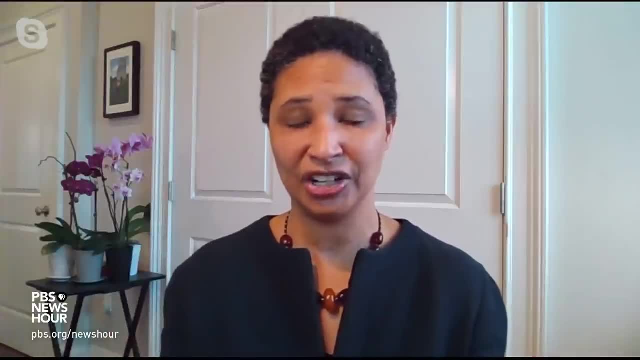 recommending that every teacher in every school teach history civics the same way. LISA DESJARDINS- Exactly, That's right. What we are doing is really issuing an invitation to the nation's community of educators to join a process of experimentation. We are not saying: here are the answers, sort of from. 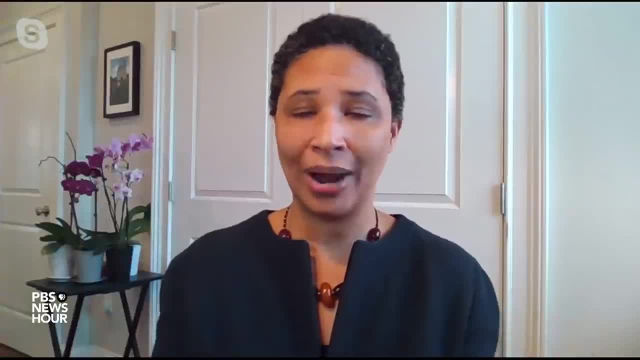 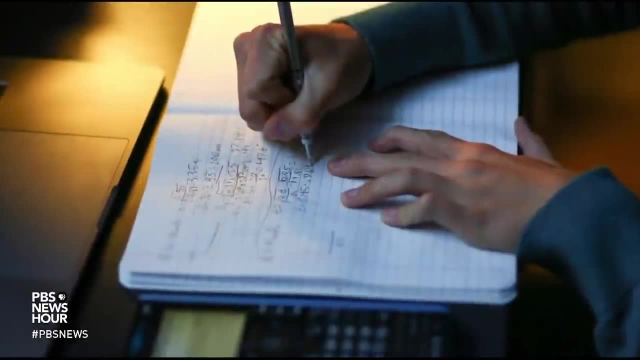 on high about how you should teach. Instead, we're saying: here is a set of questions that every learner should have the chance to encounter over their K-12 education, And we are proposing some design challenges. For example, how can we? 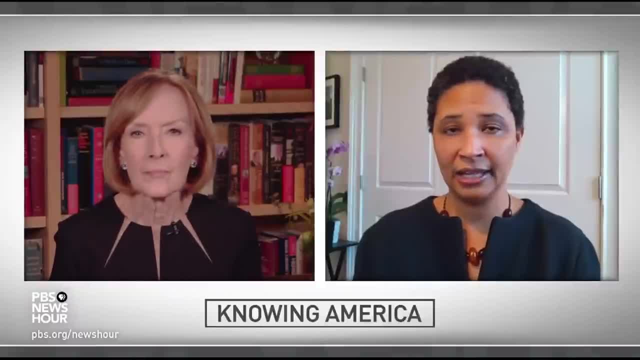 LISA DESJARDINS- narrate our history in ways that are both clear-eyed and honest about our failings, but without falling into cynicism, and appreciative of our achievements, including the founding, but without tipping into adulation. 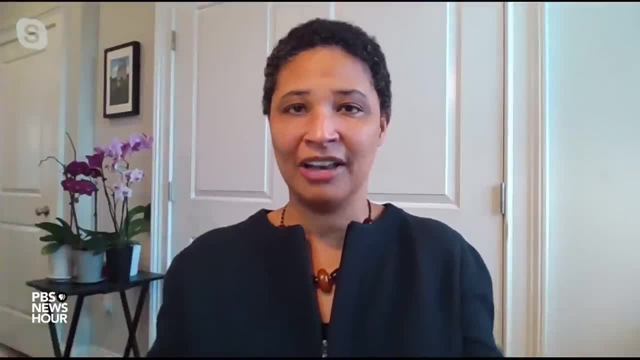 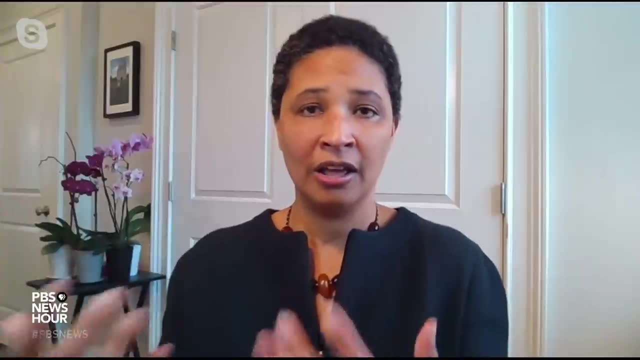 So those are some parameters, guardrails. Now here's an invitation: Community of educators, let's experiment. What kinds of histories can we tell within those parameters? How can we explain the value and purpose and functioning of a constitutional democracy within those parameters? 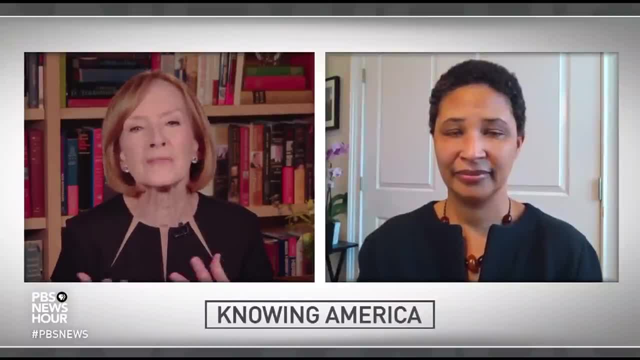 JUDY WOODRUFF. So what would some of these new ways of teaching history and civics, what would they look like? I mean, if it's not all going to be exactly the same, there are going to be some things in common. 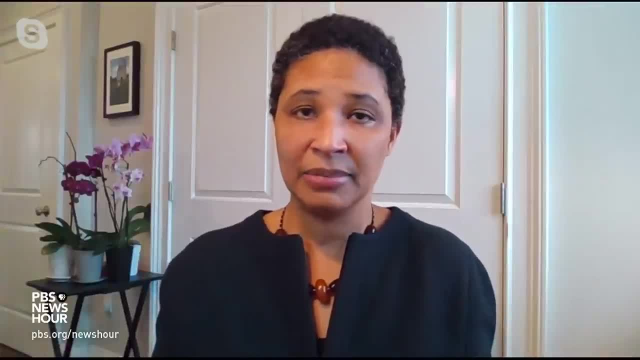 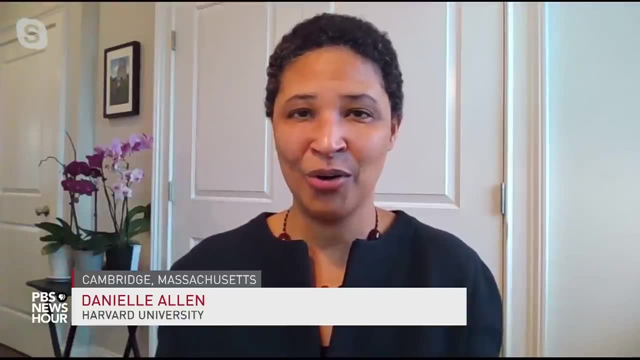 LISA DESJARDINS- Absolutely. Our hope is that everybody starts to use the same set of questions, And these questions are history questions and civics questions. To give you an example, if you look at state standards now, very often what you will see, 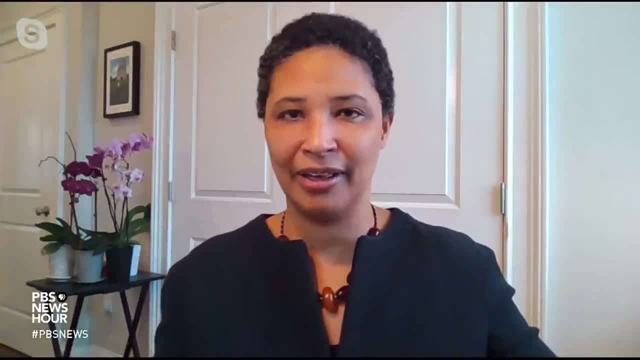 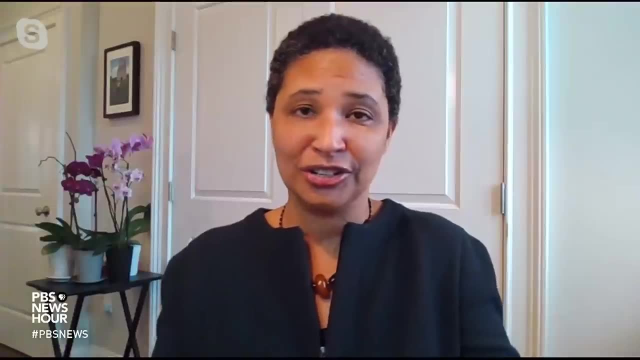 is a list of names and dates. so the Boston Tea Party and Shays' Rebellion, three branches of power, for example, or three branches of government, And we're suggesting. instead, we want to ask questions. So, when you're thinking about the American Revolution, what were the perspectives that? 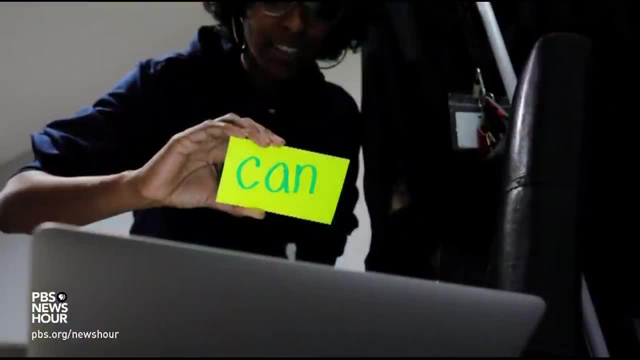 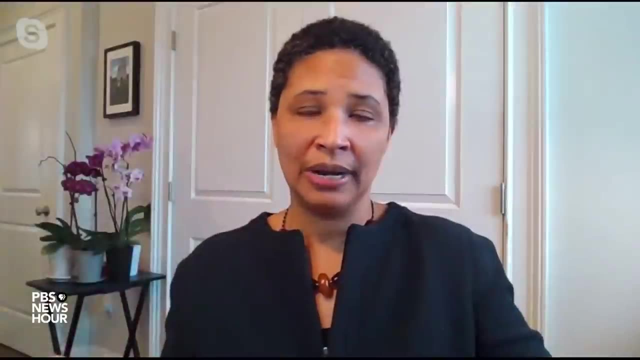 the colonists that indigenous Americans, that free African-Americans and enslaved African-Americans had on the British government? You still have to learn a lot of stuff to answer that question, but the goal is to engage students in a process of inquiry, working with primary sources to really help them dig into a broad understanding that integrates. 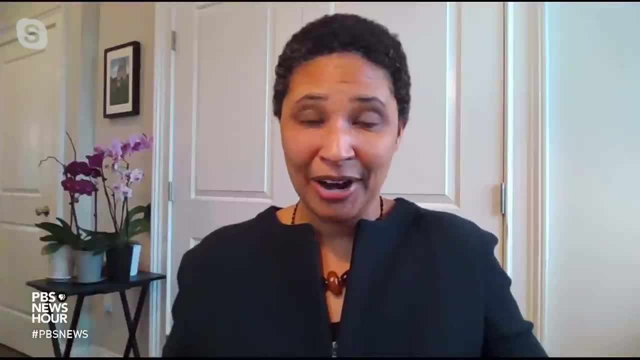 perspectives. We also ask civics questions. How do we define fairness? What are the different possible ways of defining fairness? What are the different possible ways of defining fairness? What are the different possible ways of defining fairness? How does fairness come into our lives and 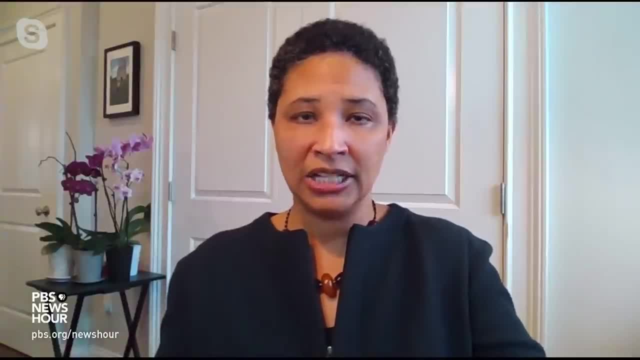 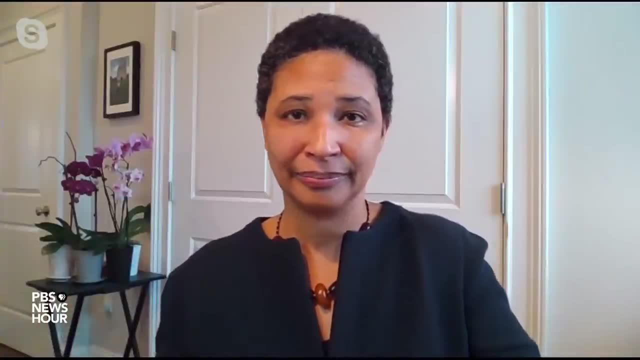 our communities and with one another, And so it's really about engaging students in those hard questions and debates and then working hard on how we debate productively with each other- JUDY WOODRUFF And with Danielle Allen, with the thousands of school districts around. 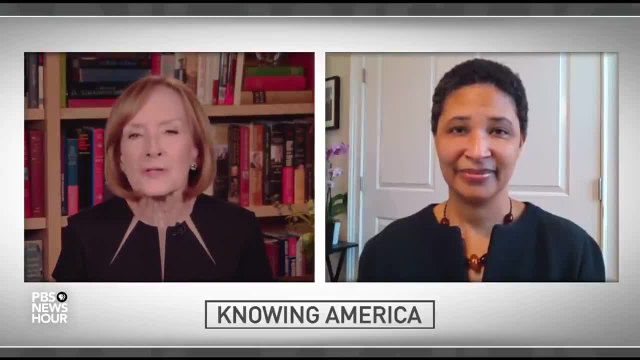 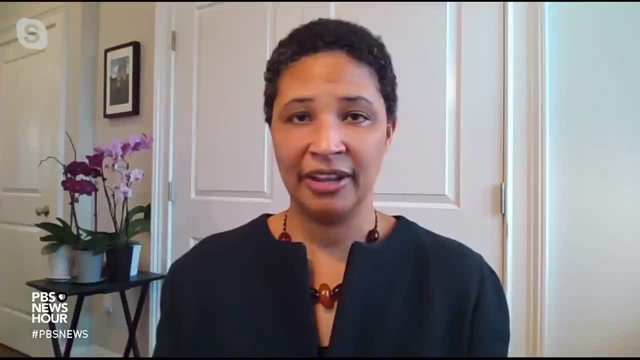 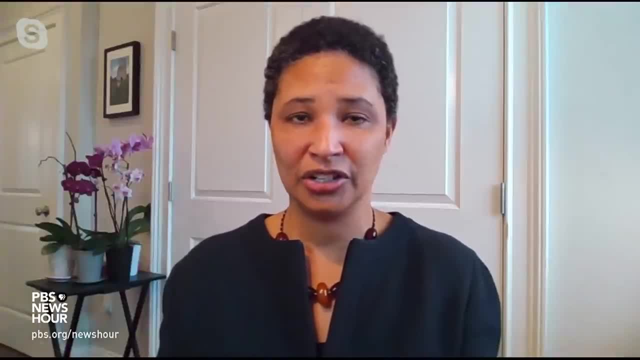 people working on this: educators, scholars, practitioners. We talked to parents, We talked to students. We have a remarkable array of civil society organizations that are contributing to this and again, from across the political spectrum. So, for example, the Bill of Rights Foundation is a supporter of the work. The American Federation 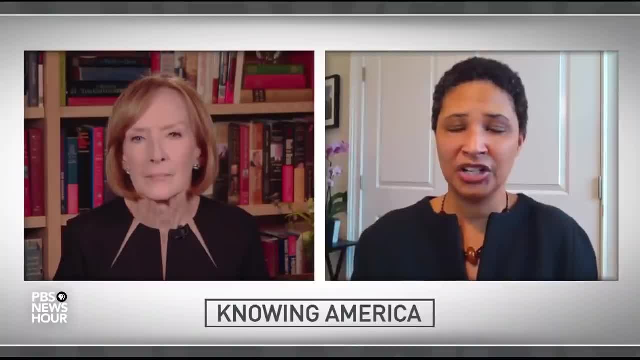 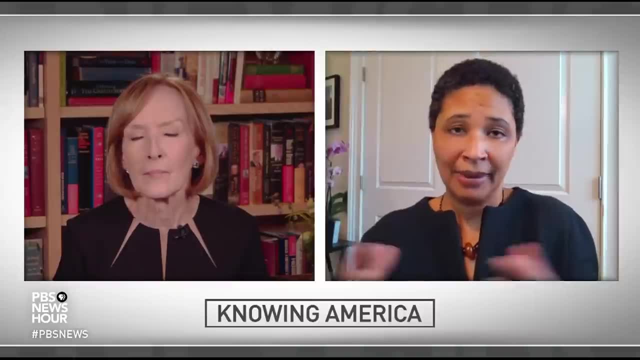 of Teachers is a supporter of the work For implementation. our argument is on behalf of what we call collaborative federalism. There is a role for every part of our system, But at the end of the day, yes, you're right. 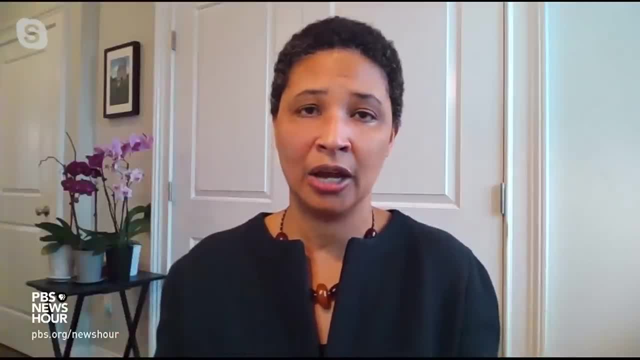 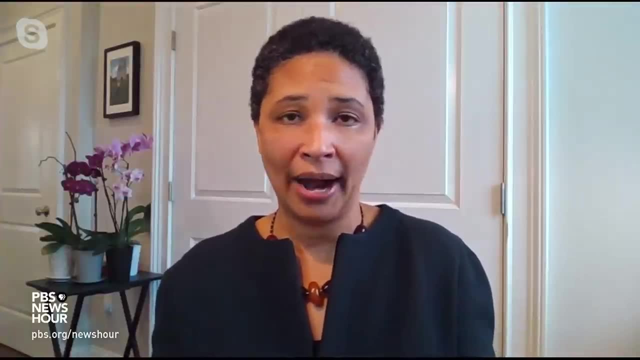 It's at the local level that civic learning is really going to take root. So we argue that schools should create civic learning plans. We do recommend that states should require this of schools. The federal government, we think, has a role in supporting professional development and 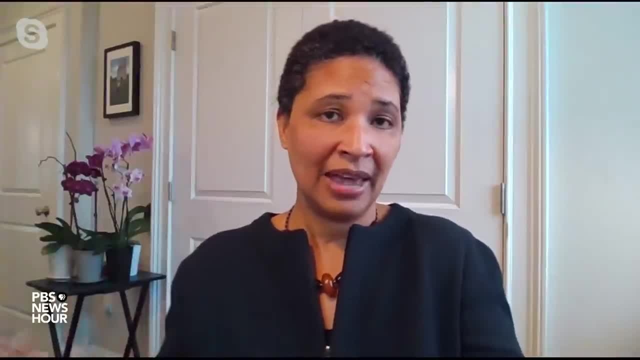 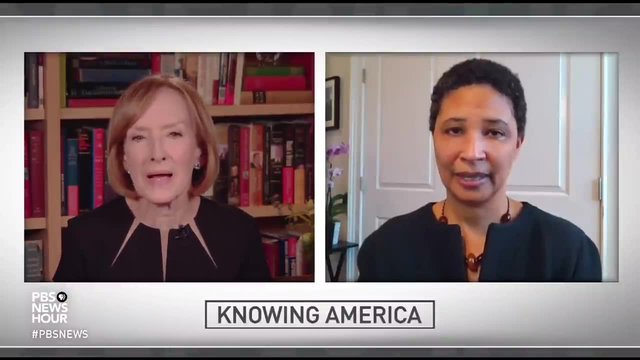 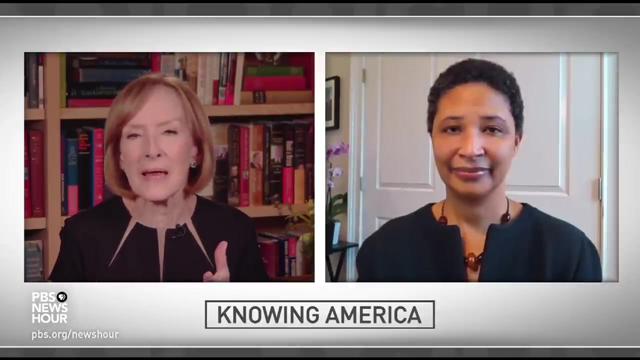 investing in diversifying the pipeline of educators, investing in innovation? JUDY WOODRUFF, The New York Times. Some of civics education we know was pushed out in the desire to improve STEM, so-called STEM education- Science, technology, math and so on. is it an either-or thing that schools are still? 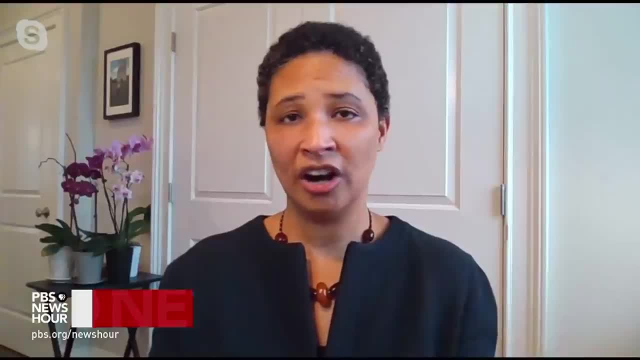 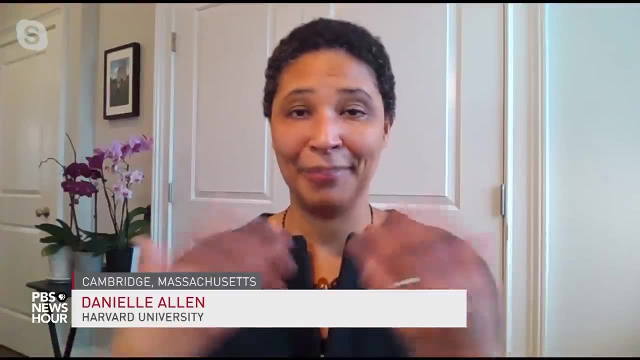 facing on this LISA DESJARDINS, The New York Times. It shouldn't be an either-or. We need our investments in STEM education and we also need our investments in civic education. We invested in STEM as a part of becoming a competitive society globally. We were thinking.